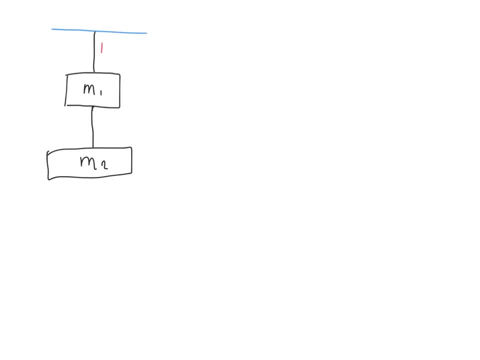 So we'll call this wire one and wire two. That way we can distinguish them and we don't have to necessarily say the same tensions are involved. But what if? then we really want to figure out, okay, what is the tension in each of these wires. 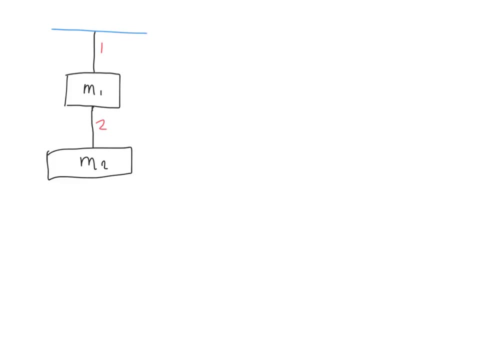 So it's probably too complicated looking at everything here together, So let's actually look at each block individually. We could look at also at the wires individually, but it's much easier to just work with the blocks. So let's look at, for example, block one. 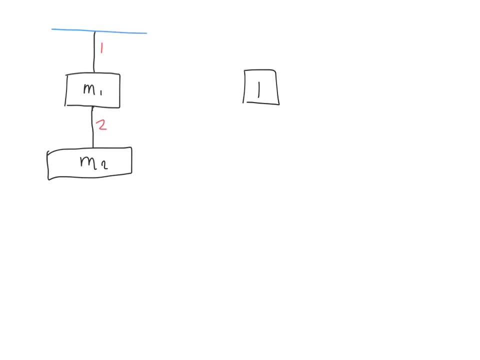 And consider the forces acting on block one, Well, it definitely is going to have its own weight downward. That's a given, as long as we're doing this on a planet with some gravity, and you probably would in your life. On the other hand, of course, we expect there should be a tension force upward. The wire is holding the tension force upward. 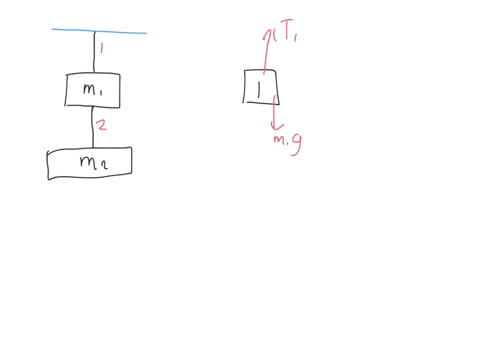 The wire is holding this thing up. On the other hand, of course mass 1 is also attached to mass 2 by a wire, so that's also kind of pulling it down. So we'd also expect there to be tension 2 acting on block 1.. So if I were to set up Newton's second law here for this block, I would 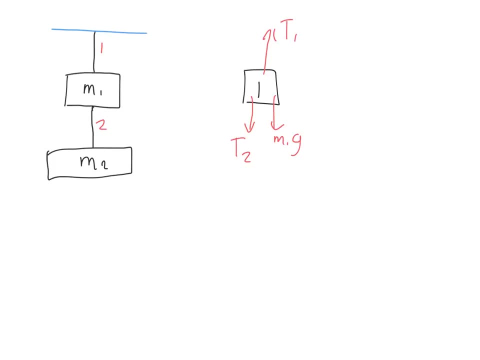 have two tension forces, That's two unknowns with one equation. I probably won't get very far starting there, but here's our setup and we can approach this. maybe in a little bit Let's also set up a free body diagram for block 2.. Again, we have its own weight. 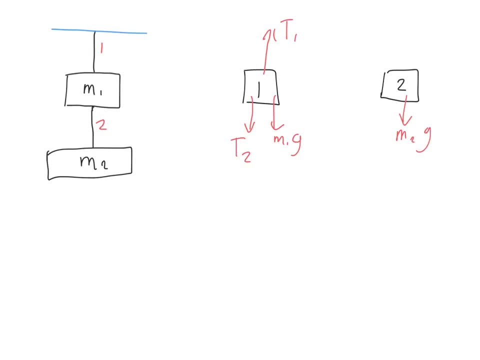 pulling it down, and in this case there's only one wire acting on it, wire 2, so there's tension 2 upward, And also do you mind the labeling I have? So this tension 2 and this tension 2 are the same. 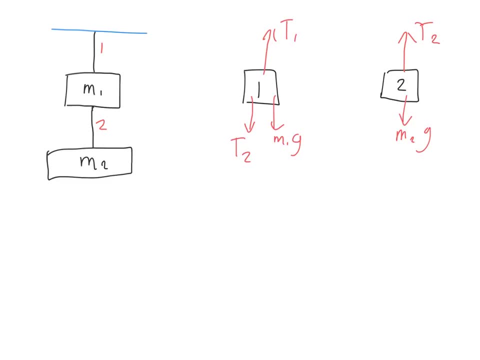 magnitude, even though they're pointing in different directions, But nonetheless the same magnitude. so this will be useful. Now, if we just have the simple case here of this being static, of everything just hanging out here, then we know there should be overall no acceleration. 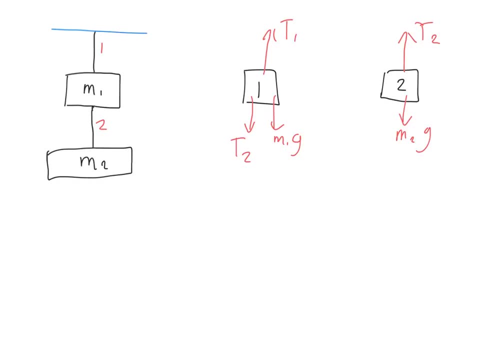 in the y direction, or even in the x direction, We'd expect as well. So we know that the forces need to balance out, which will be extremely helpful. So I had mentioned that if we try using Newton's second law on this, block immediately. 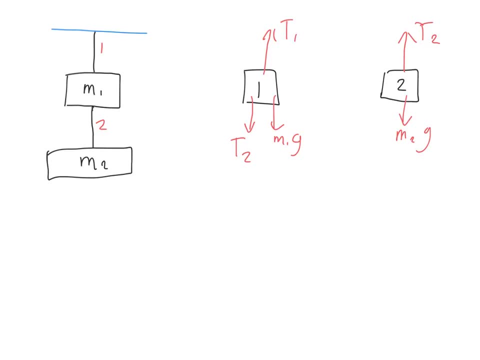 we'll have two unknowns in it, tension 1 and tension 2.. So that might be a little bit too hard. to then figure things out, Let's start with this block, where it's as simple as can be. So let's do the sum of the forces on block 2 in the y direction. 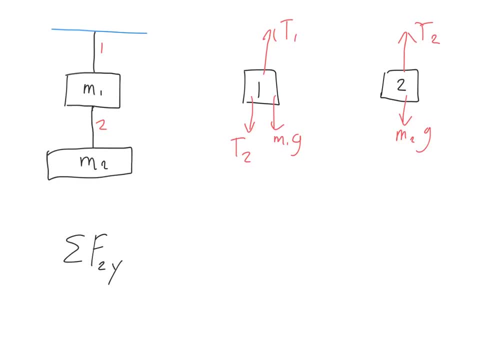 In this case we're going to say that positive y is up and the x direction. there's nothing going on there, So we'll just ignore that for now, since there's nothing to play with. So with this setup, tension 2 is in the positive direction, Weight is downward, so in the negative. 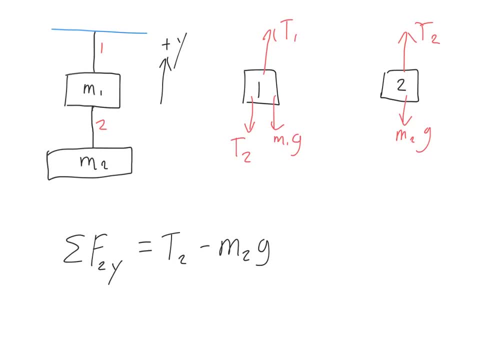 direction. And again, since this is not accelerating, the forces balance out. Some of the forces should be 0. Aha, So with one step of algebra, I see that tension 2 is just the weight of that block. Not too bad, Not too bad, Let's give ourselves a little bit of space now We'll set that. 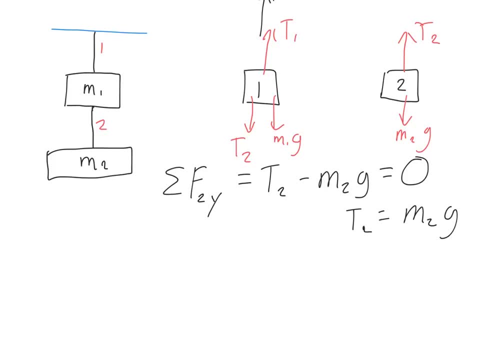 result over here And we can do the same thing then to talk about the sum of the forces on block 1 in the y direction. So in that case we have tension 1 up, Tension 2 downward acting on that block And the weight of that block, And again we're. 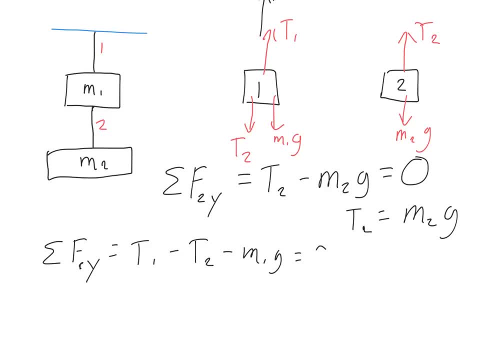 talking a static case, so this should just be summing up to 0 again. So I can solve for T1 with just a little bit of algebra, And I see that T1 is equal to tension 2 plus m1 g. We already solved for tension 2.. I can plug that in, And so I actually 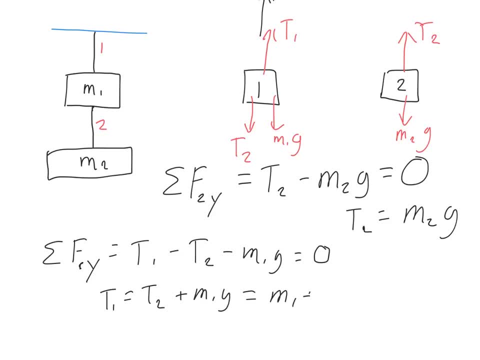 see that With a little distributive property I can write this like so: And if you were to first guess what the tension should be, it kind of makes sense that tension 1 is effectively holding up both blocks. And that's exactly what we see here, that tension. 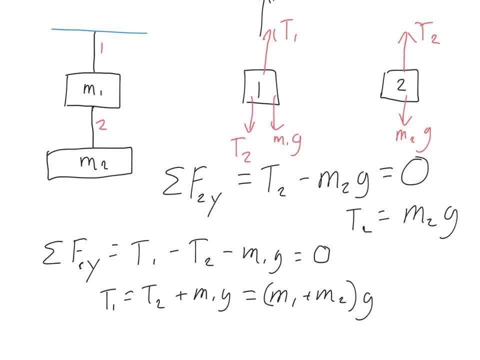 1 is holding up both masses here, the weight of those two masses connected together. Not too bad overall. That's not too difficult, And this, of course, was for a static case, So the correct answer was 0.. There we go. Great, We're done here. OK, Thanks, Thanks, Thanks. And now let's talk about the termination process. So we're going to have one more example. So I just want to touch up at the end. I'm going to go over to the bottom right of the table. 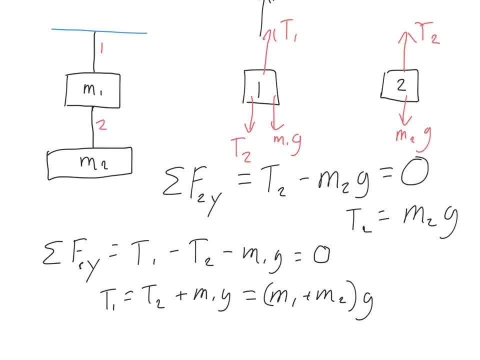 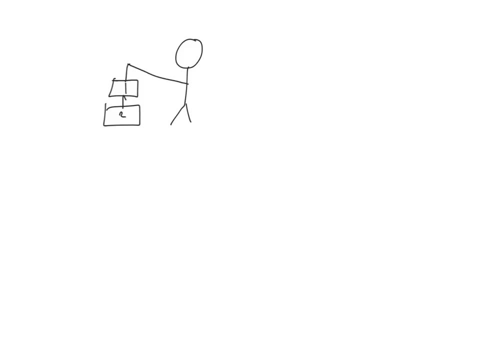 case? Alright. then what if we wanted to complicate things a little bit In this scenario? instead of hanging the masses up, I'm going to hold them, and not only I'm going to hold them in place, but I'm going to lift up all these masses and 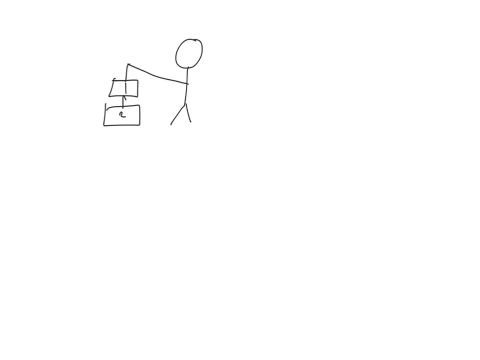 accelerate them upward. So I'm working my muscles and let's say I give an acceleration to this system of one meter per second squared. So the blocks are going to move up and they're going to accelerate upward for whatever period of time. So at this instant we can look at the tension here. We still, ultimately, 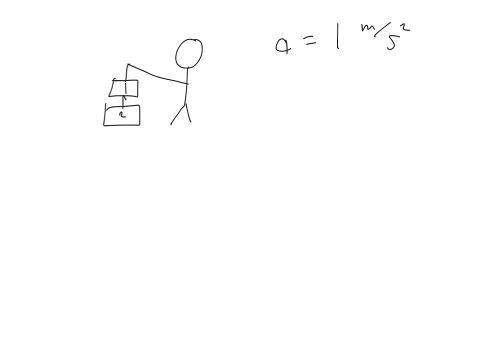 have the same free body diagrams. the exact same forces are acting on the blocks. So for block two, there's only two forces: its weight and its tension. On block one, there's only three forces: tension up, tension down and its own weight. It's the exact same sorts of things, but now. 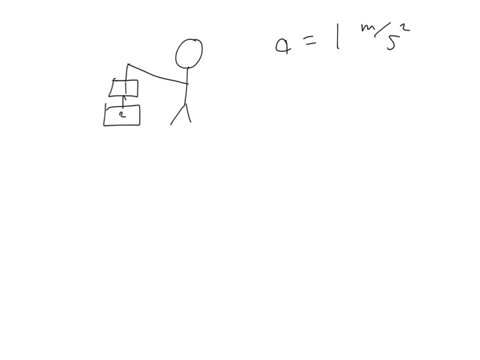 there's acceleration involved. So let's take a look at that scenario. So let's again do some of the forces on block two in the Y direction, and again we'll still say that up is positive Y and I'm accelerating upwards so it's a positive. 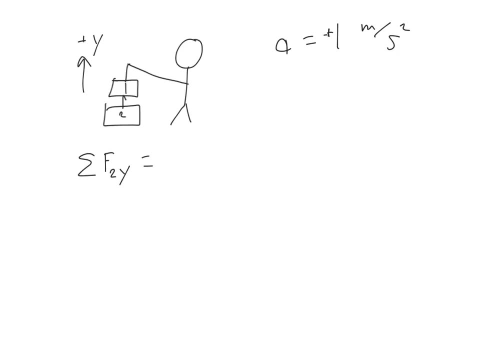 acceleration. So in this case we still have tension to upward, the weight of block 2 downward, and in this case, from Newton's second law, the sum of the forces is mass times acceleration. Nonetheless though, I can still do the same sort of algebra and solve for T2 algebraically, and I can also do a little. 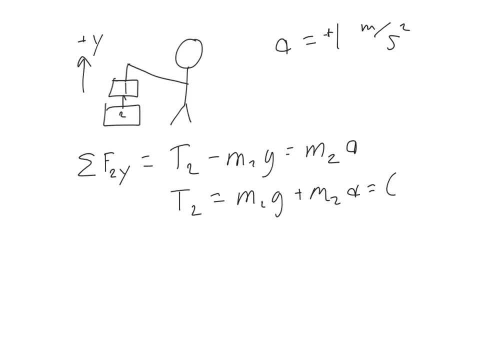 distributive property and make this a little bit cleaner. so I would have G plus A times M2, just to make it look a little cleaner. Alright, and I can also set up some of the forces on 1 in the y-direction. We'll have tension 1 up. 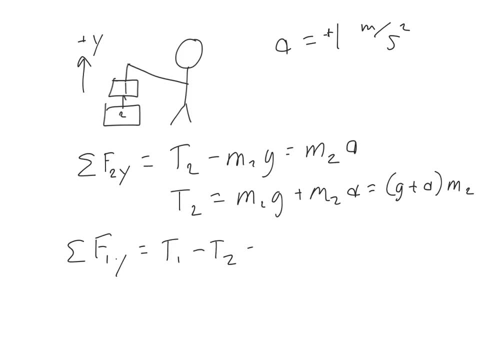 using the same notation I had before: tension 2 down. weight of mass 1 down equals that mass times the acceleration. and notice the labeling I have chosen: mass 1, mass 2, the sum of the forces on 2, sum of the forces on 1.. One thing: you definitely want to be careful, don't just 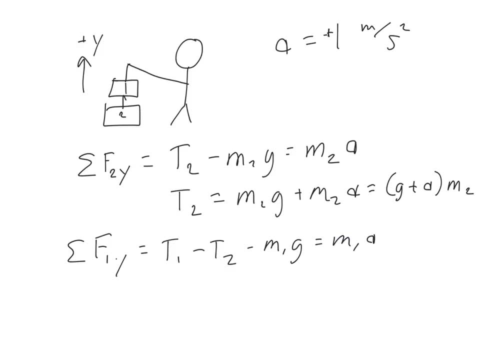 write mass here. you want to specify which mass you're dealing with. you're doing the sum of the forces on body 2, you need then the mass of body 2, just for clarity. Okay, so again, let's just solve for T1 algebraically, and we see. 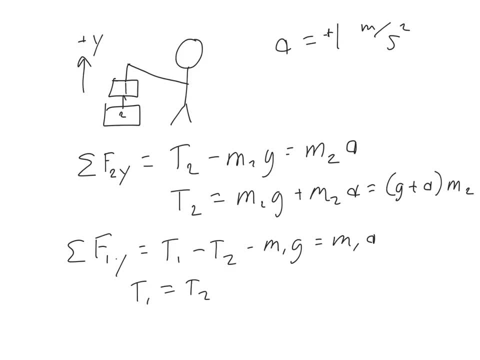 that would just be T2 plus, and I'll do the same sort of distributive stuff I did earlier where I have plus a m1.. Okay, and you see that I could also then plug in what I had for t2 here doing that, and what I will find is I can do a lot more of the same sort of. 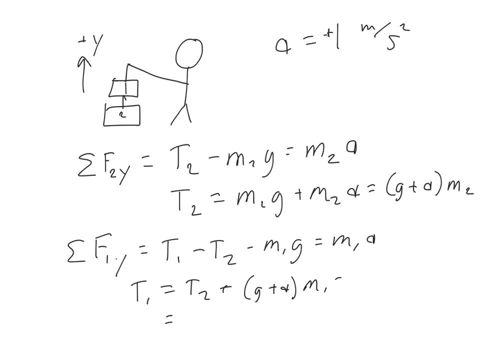 distributive stuff here Make it clear. so I will have g plus a m2 plus g plus a m1.. So again I could do distributive property things and find g plus a times m1 plus m2.. So again, what would this mean? So again, what would this mean? So again, what would this mean? So again, what? 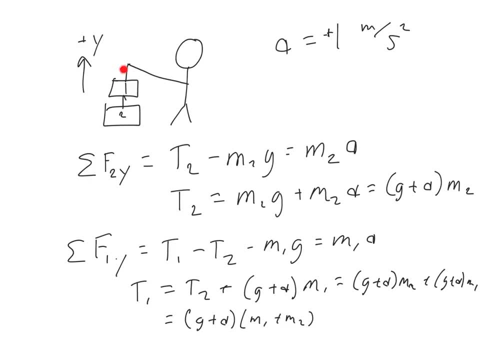 would this imply? Oh well, that the tension here has to again lift both masses, and so it basically has to be strong enough to hold up the weight of those two masses. the g term, the weight term, then, and then how much it needs to. 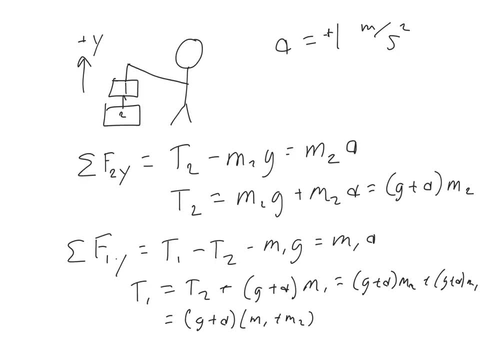 be accelerated, And from either setup what you would expect is that this wire is under more tension than this wire. We see that t2 is just m2 times g plus a, but for tension one it has to as both mass terms. so it's always going to be. 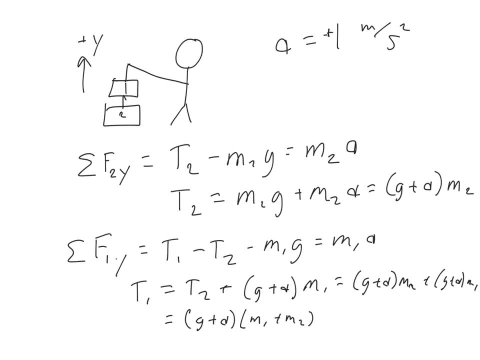 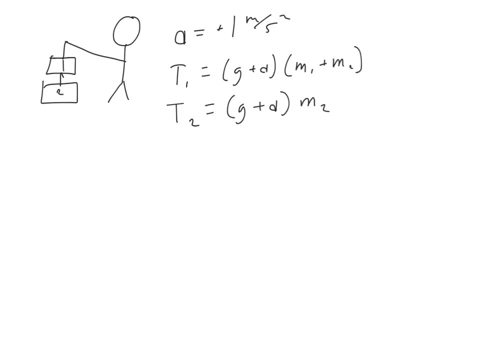 larger. So if you were to accelerate this thing, if you were to expect either of these wires to break, you would think the first one would break before the second one, since the first one's holding up with a lot more tension. So we had done. 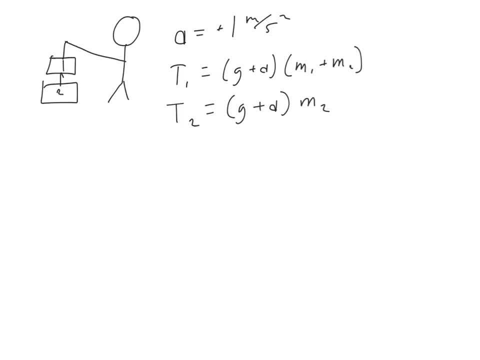 everything algebraically, but let's plug in some numbers just to make things absolutely concrete. Let's say that mass one is just one kilogram. Mass two, on the other hand, we'll say, is five kilograms, just to have some numbers, And we'll keep the same. 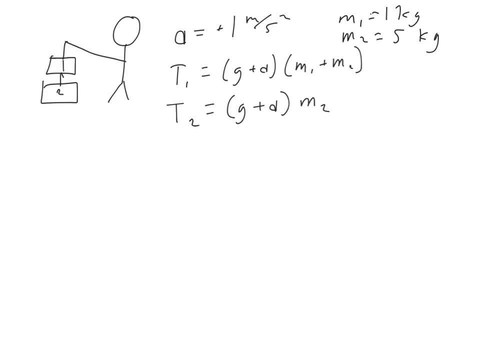 acceleration. we'll assume this is on Earth. so the acceleration due to gravity is nine point eight meters per second squared, And so if we do that, we're going to find then that tension one is going to be nine point eight plus one times mass one, one plus mass two five. So this is 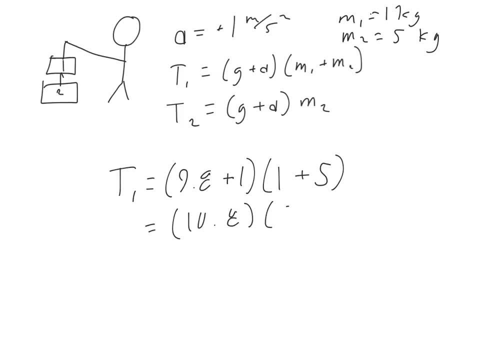 ten point eight times six, which equals sixty four point eight newtons, And tension two, just plugging in our numbers again nine point eight plus one, and then just the mass of two, which is five. Ten point eight times five, That equals fifty four point zero newtons. So here a clear case, then, where tension one 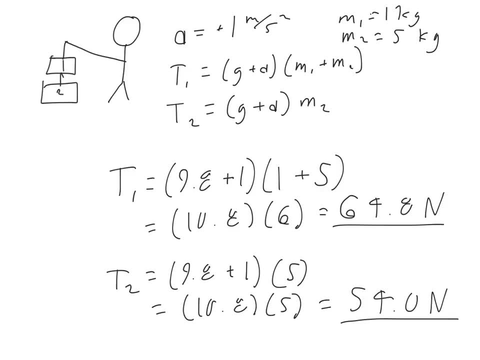 is greater than tension two and should always be, unless somehow you find some negative mass blocks which I will tell you are very, very hard to find, and if you do, there's a Nobel Prize waiting for you. So, for procedure, the way you find the tension force is in many ways much like you do for finding the normal force. You 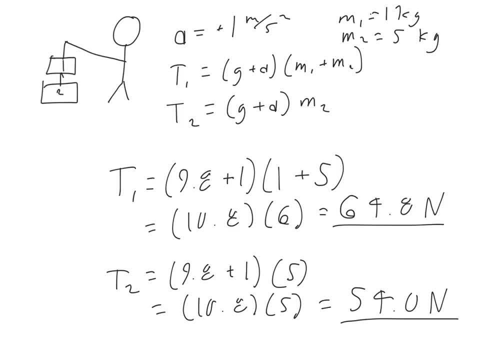 set up your free body diagram and then use Newton's second law to do the sum of the forces equaling the mass times acceleration of the body in the direction the tensions are pointing. It could be a static case, in which case there's no acceleration, or could be someone lifting up the whole system and